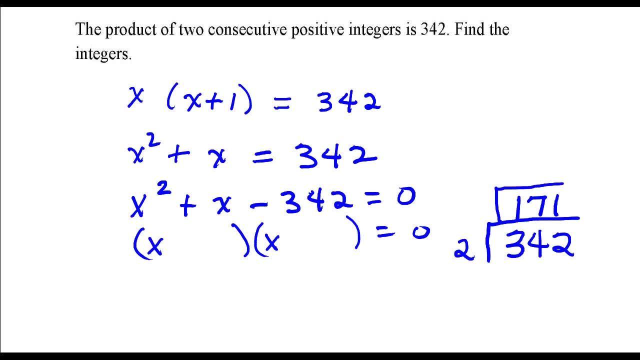 And 171 is no longer divisible. It's not divisible by 2,, but it is by 3.. And that's going to be 57.. 57 is divisible by 3.. 57 is divisible by 3.. 57 is divisible by 3.. 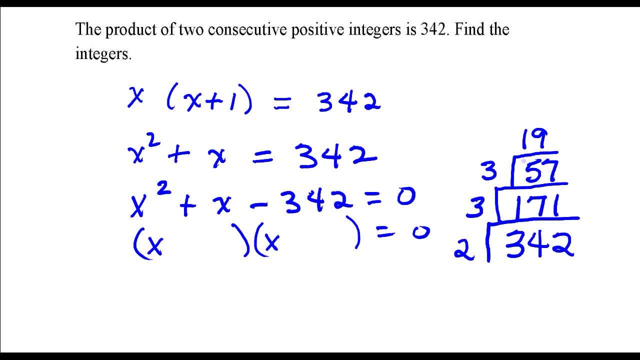 And now I can stop there, because the quotient is a prime number. So 342 is 2 times 3 times 3 times 19.. So if I multiply these three numbers together, that's 2 times 3 times 3,, that's 18.. 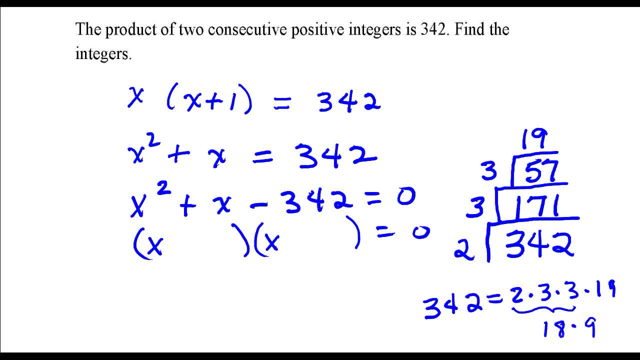 So 18 times 19.. So 18 is 342.. Okay, so let's try this: Put an 18 here and a 19 here. If I multiply these two together, I would get 342.. One of these needs to be negative and one's positive. 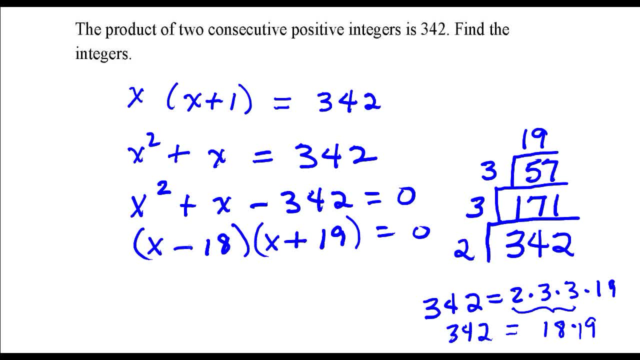 So this one needs to be positive, This one's negative. So let's check this. Negative 18 times positive 19.. That's a negative 342.. But if I add negative 18 and positive 19 together, I will get 1.. 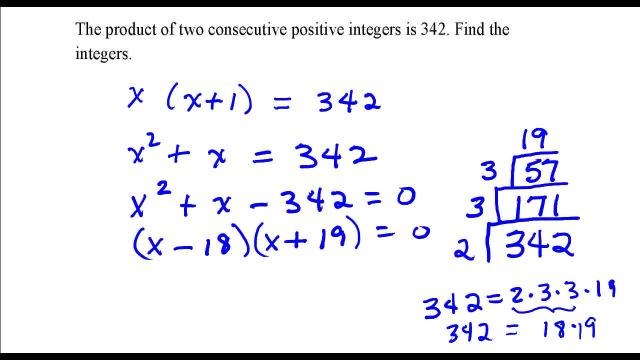 So that's the correct factorization. Now I'll go ahead and solve each of these: X minus 18 equals 0. So X is 18.. And this one X plus 19 equals 0. That gives me X is equal to a negative 19.. 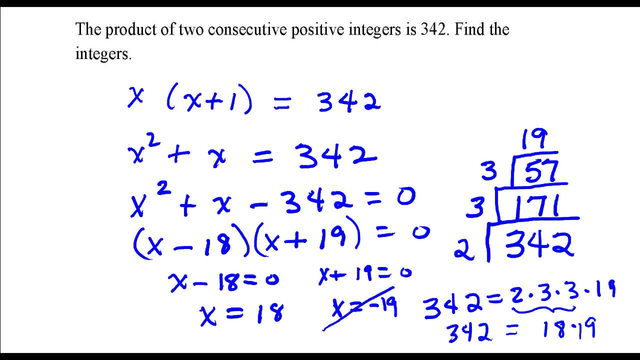 I'm going to go ahead And throw this one out, because in the context of the problem, the first sentence says: the product of two consecutive positive integers is 342.. So negative 19 is not positive. So that's why we throw that out. 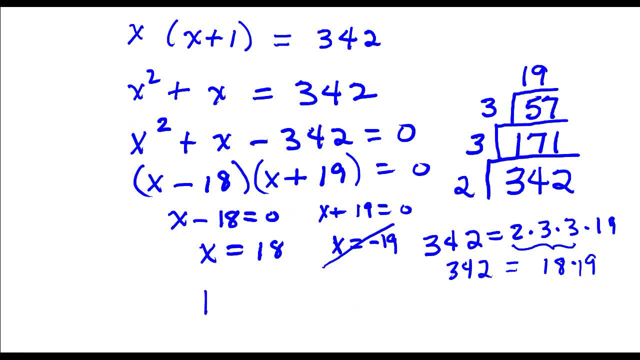 So those two integers would be 18.. And then the next consecutive integer would be 19..